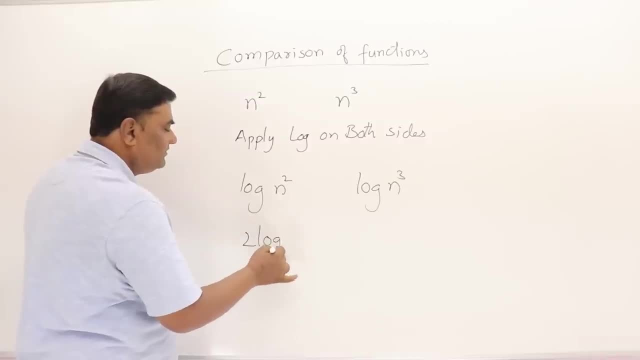 Then this becomes 2 log n And this becomes 3 log n. Now, this is log n, This is log n. They are same only, But this is 2 times, That is 3 times, And definitely this is less than that one. 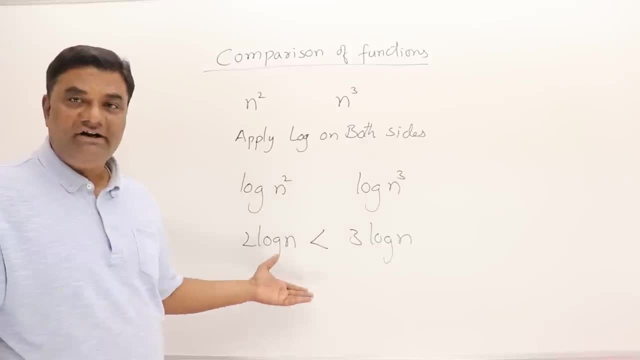 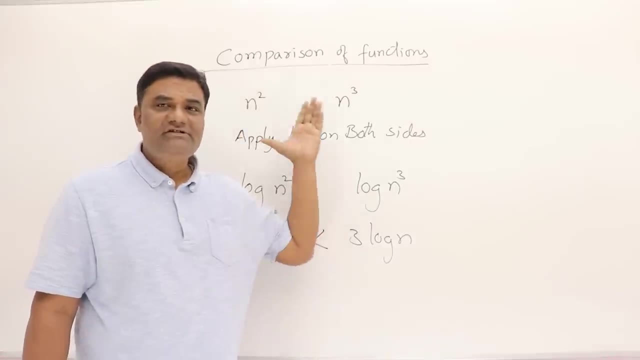 So second method is: apply log n. So let me go on both sides to find out which one is smaller and which one is greater. So if you have some complex functions, then this is useful. This is a known function only, So I am taking a known thing to make you understand what is the method of checking them. 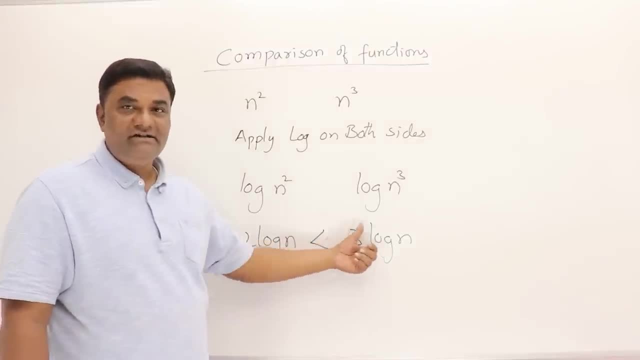 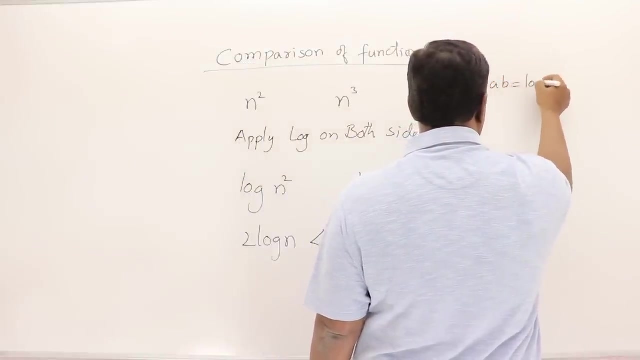 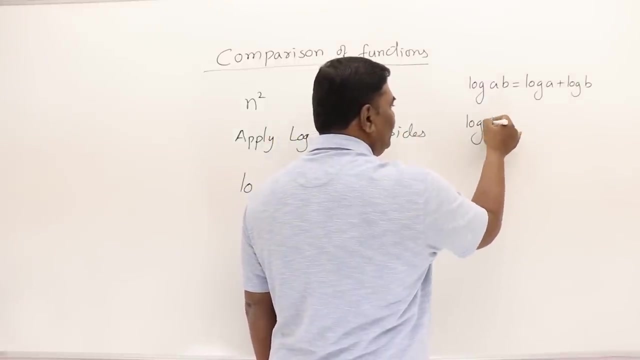 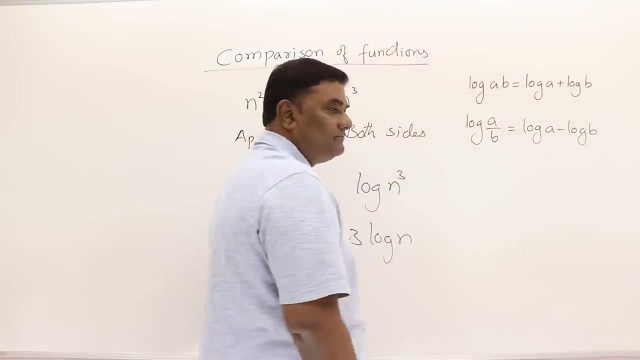 So 2 log n. So I should check exactly 2 log n is less than 3 log n. So for applying logs you should know some formulas for log. So let me write some formulas here. log A into B is log A plus log B. Log A divided by B is log A minus log B. Log A to the power. 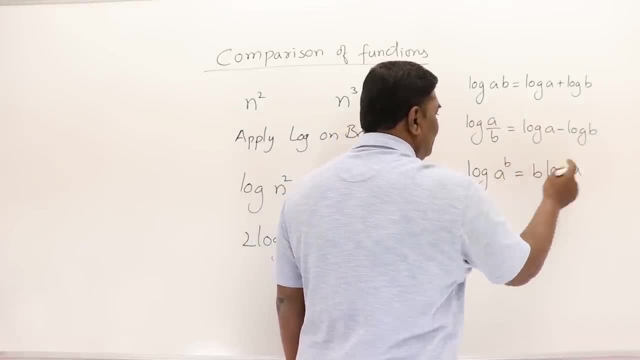 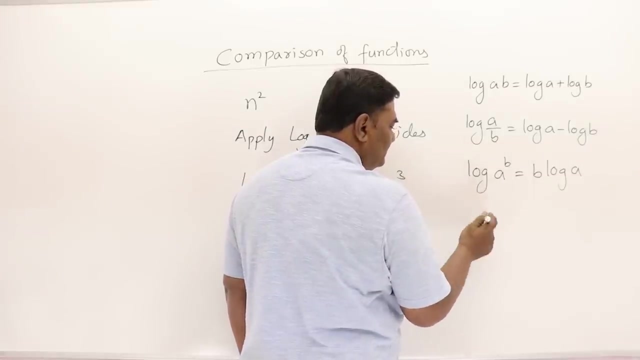 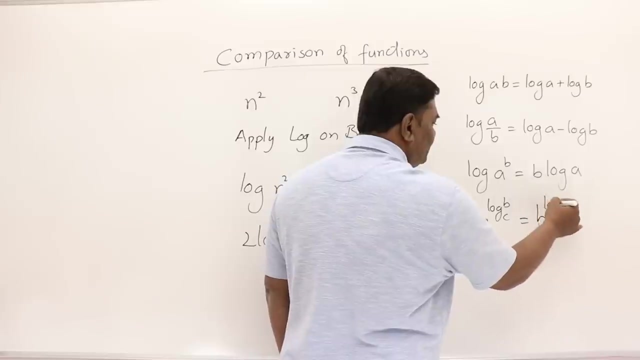 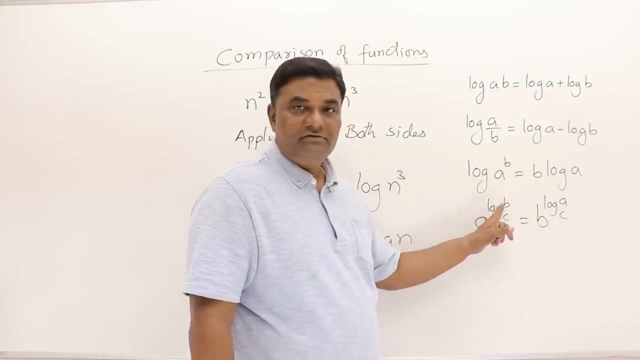 of B is B log A. If you have any power here, that will come this side. It will become coefficient. A power log B base C. is B power log A base C: Right, So this log value can come as a base here if it is in power. 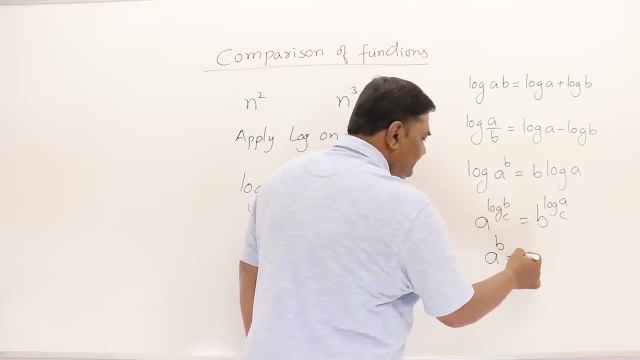 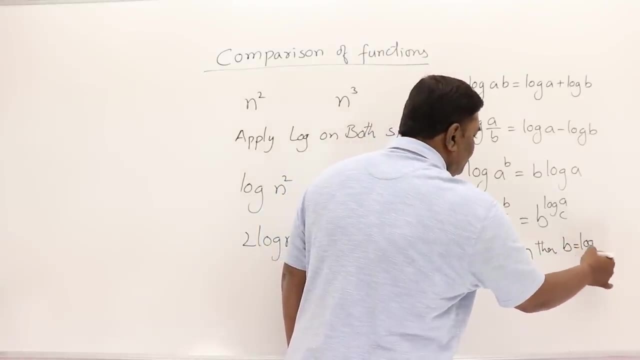 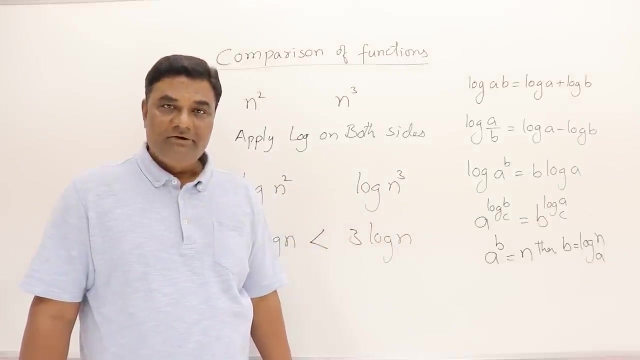 And A power B is equals to N, Then B is equals to log N, base A. These formulas must be helpful for solving log problems. So now the objective is to compare functions. So I will write a few functions and let us compare them and find out which one is greater. 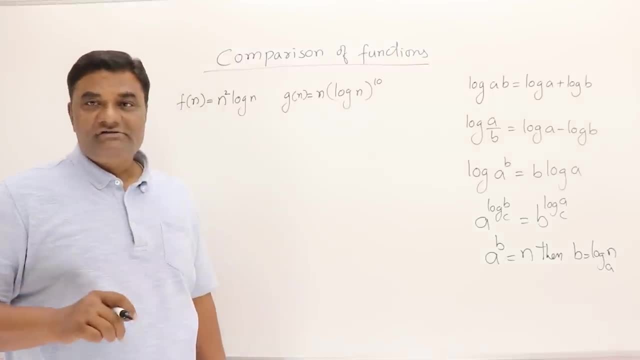 and which one is smaller. Here I have two functions. Let us find out which is greater. Compare them. So F of N is N square log N. G of N is N log N whole to the power of 10.. So power of 10 is greater. So it looks as if that is greater than this one. 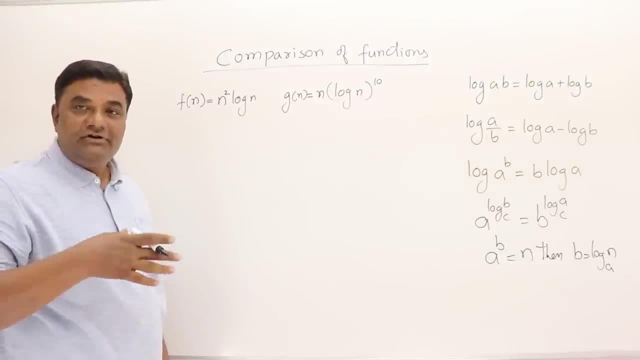 We know N square is greater, So now it will confuse. So if you are unable to judge which one is greater, right. If you are able to judge this, Then no need to do anything If you are able to judge it perfectly. 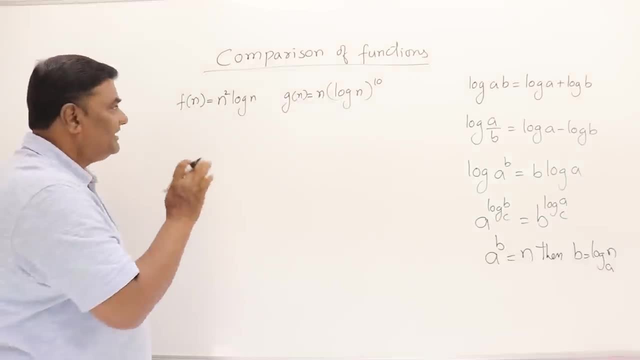 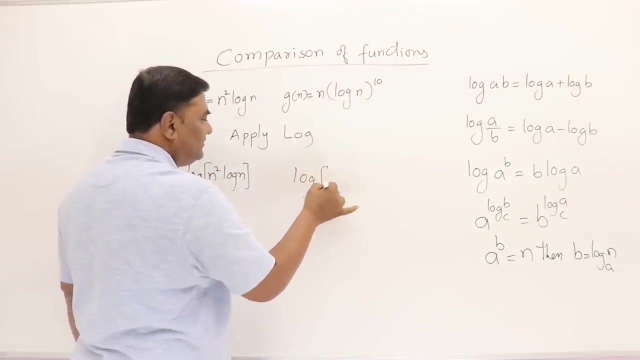 Then let us compare and find out by applying log. Apply log. So this is log N square, log N, And this is log N, log N. This is power 10.. If you open this one, This is log N square plus log of log N. 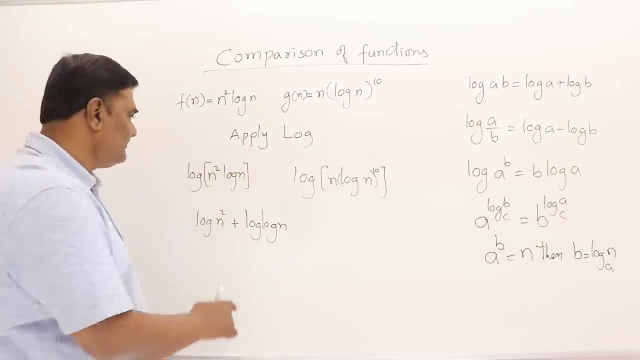 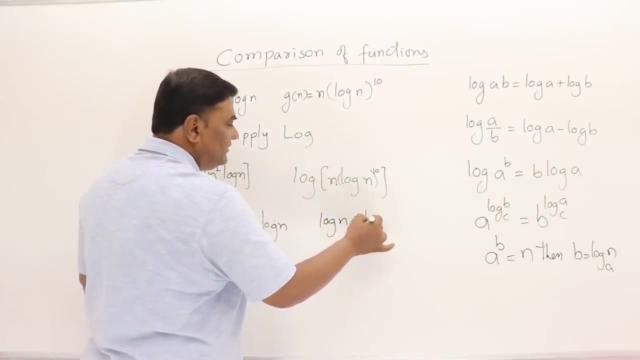 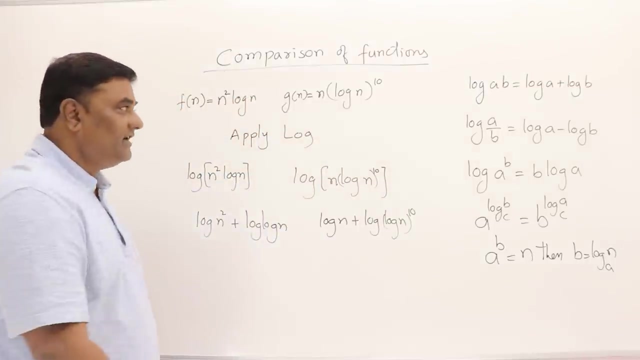 As we know, log A into B is log A plus log B. So log A plus log B. Now this side, it will be log N plus log of log N, whole to the power of 10.. So this is log N. We have used first formula. 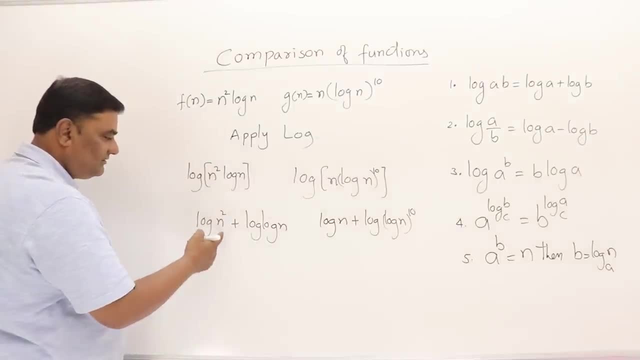 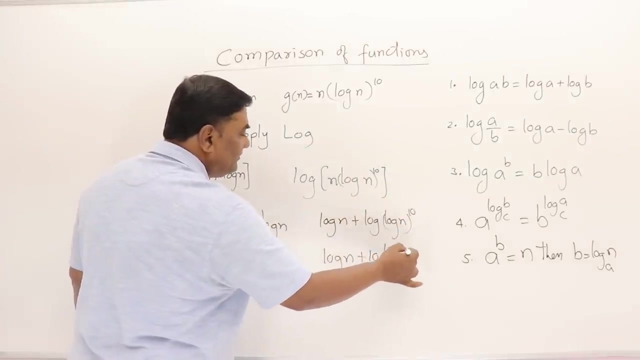 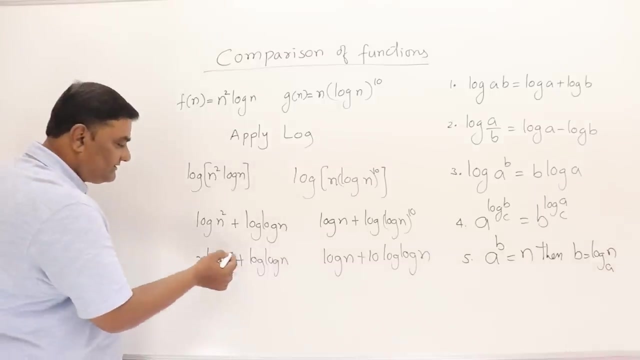 Now using the third formula there, This becomes 2 log N plus log of log N, And this is log N plus 10 is in power. So 10 log of log N. Now check this. This is the bigger term. This is the bigger term on that side. 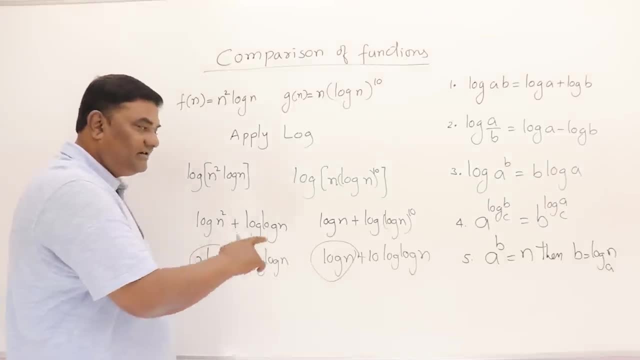 Now, if you check two bigger terms, This is 2 log N and that is just log N. So definitely 2 log N is greater than this one. Now that is a 10 N log of log N And this is just log of log N. 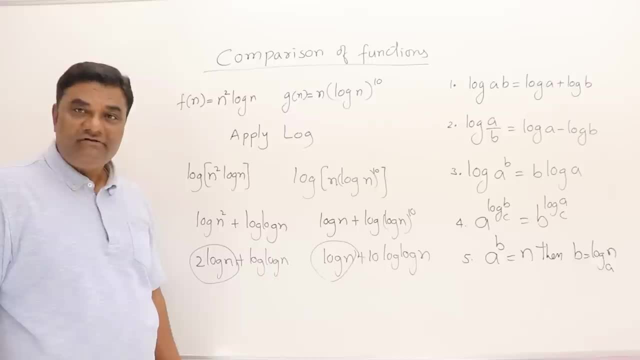 So that is a smaller value. Log of log N is a smaller value. You can take it as 2 rupees Some paisa And 1 rupee Some paisa. So paisa is smaller than rupees Right. 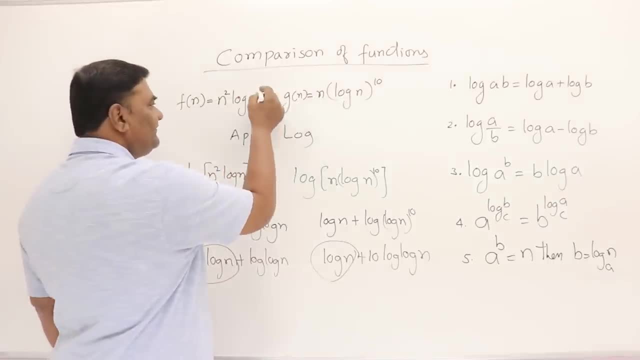 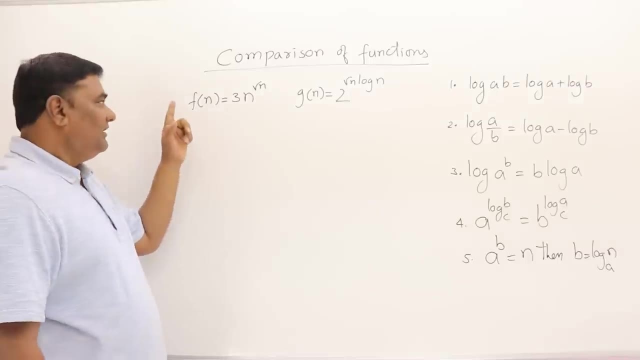 So this is greater, So this function is greater than that one, So this is greater than that one. Now, second example: F of N is 3 N power root N And G of N is 2 power root N, log N. Let us compare. 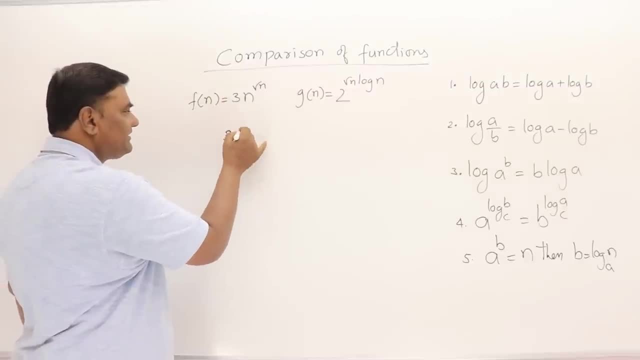 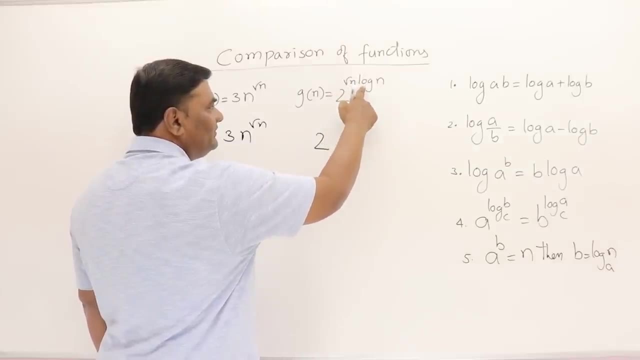 So for comparing, I will first write it as it is: 3 N power root N And this is 2.. And this is log N, root N, log N. So if you apply this third formula, Then this can also be written as N power root N. 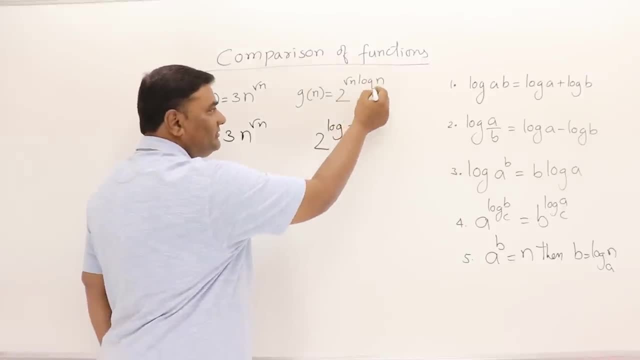 And this is base 2, only Log base 2.. Here it is base 2.. It is always By default, always it is base 2.. So it is 2 power. log N power N. Right N power N. 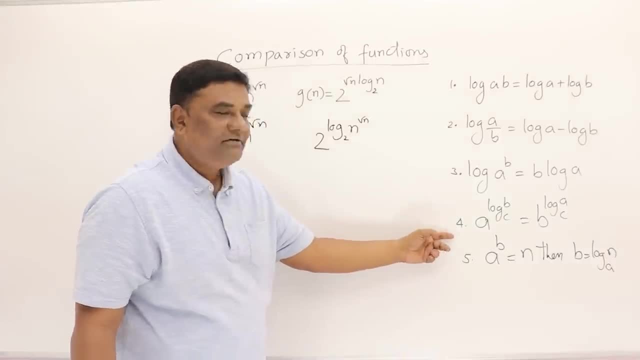 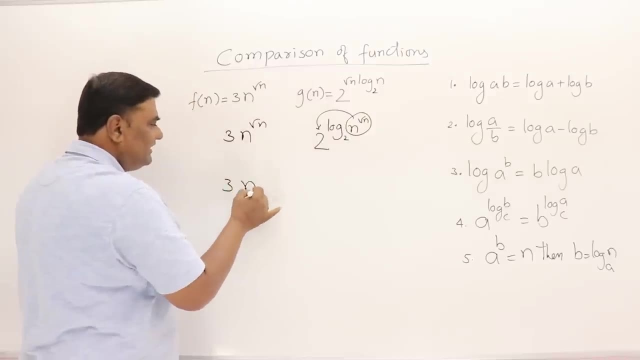 Now By using the fourth formula. Fourth formula, What I can do is This: I can interchange with this one, So this will be 3 N power root N, And that N power root N comes here And hold to the power of log. 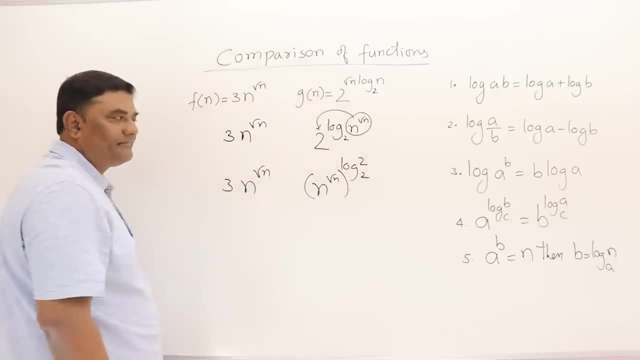 This 2 goes there, So 2 base 2.. Log 2 base 2 is 1.. So it is power 1.. So what is the answer? 3 N root N And this is N power root N. Now I have two functions. 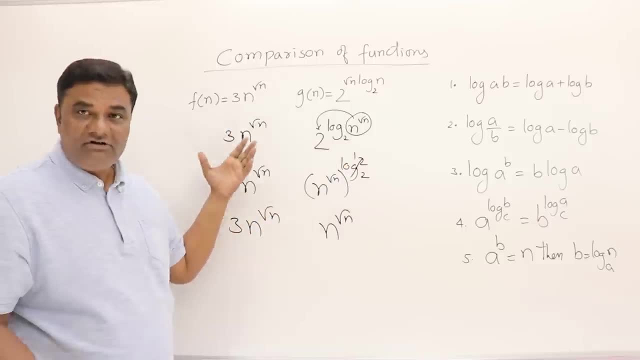 So I did not apply log Without applying log. I have not applied log on both the side, But I have used the formulas of log For solving them. Even you apply log also, you can get something. So now, what do you see? 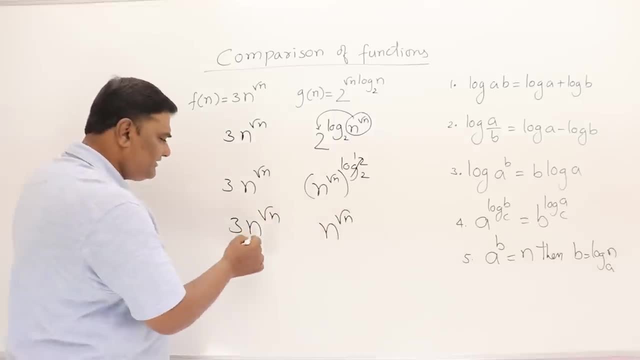 3 N power root N. N power root N. So if you see the term, They are same. This is just a coefficient. This is just a coefficient. It is just like 2 N square and N square: Who is greater? 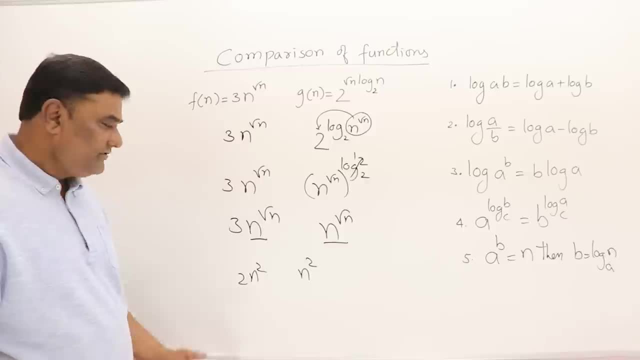 They are equal. They are equal. This coefficient is ignorable, Right, Asymptotically. they are equal. Value wise. this is greater Order of N. if you write Big O of N square. if you write Big O of N square. 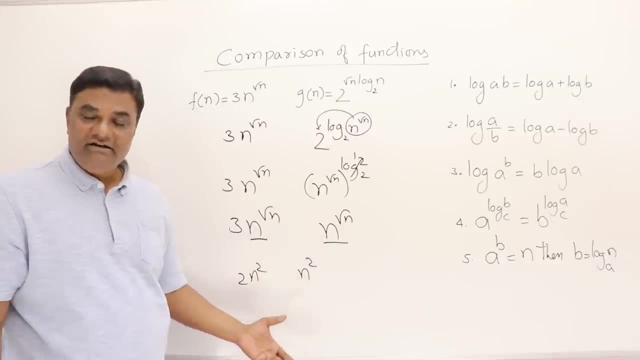 Big O of N square. Asymptotically they are equal, But the value wise this is greater than that one. So if you want asymptotic answer, Then both are equal. Both functions are equal.